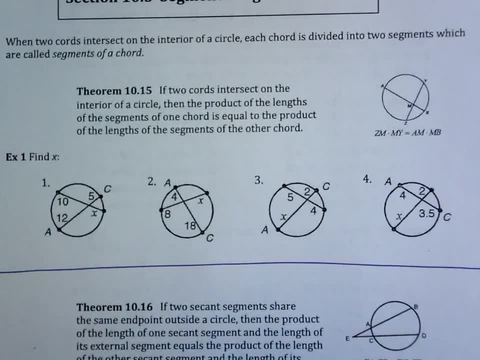 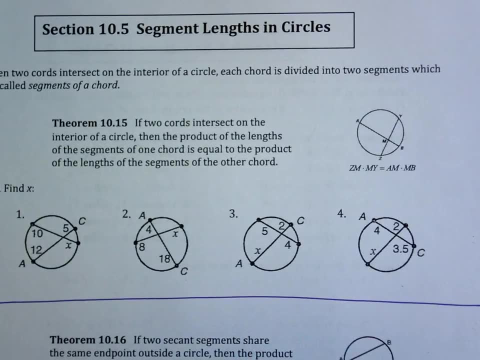 and say there's one rule for how we do all of these and then there's another rule for how we do the ones below that. Okay, it says when two chords- and it's interesting, I think this might be, I don't know, British or something. 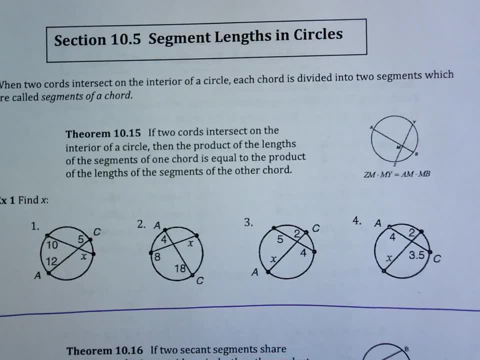 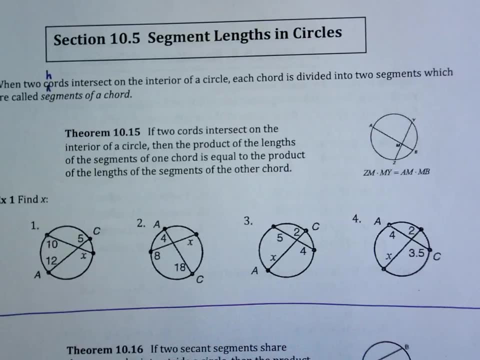 chords. there's no H. No, they spelled it right other places: When two chords H, When two chords, When two chords intersect on the interior of a circle. So it's still. the difference is still going to be where they intersect. 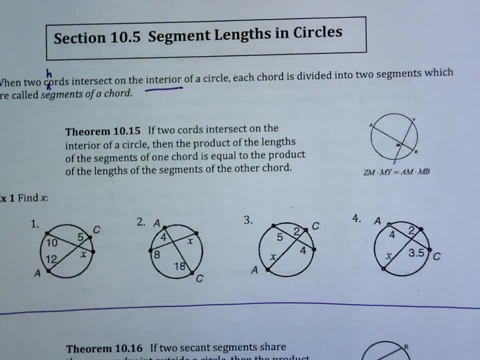 whether they intersect inside the circle or outside the circle. That's still going to be the difference, but we're not thinking about it in terms of angles, though We're still. we're just talking about segment lengths, chord lengths, segment lengths, secant lengths, tangent lengths. 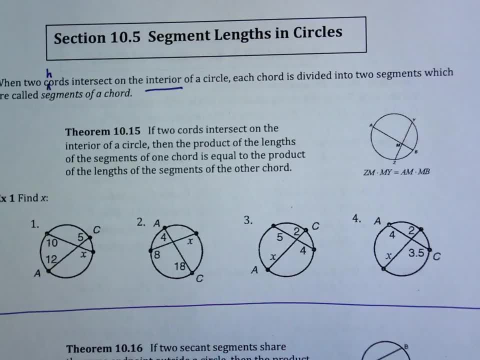 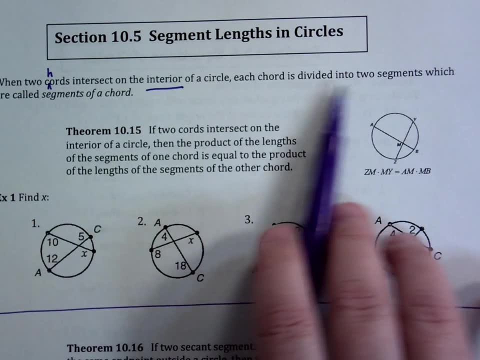 It's all segment lengths, but it still does matter. The difference is where do they intersect each other- inside the circle or outside the circle? So if they're inside the circle, each chord is divided into two segments. So in other words, they're saying, like this whole chord has two parts. 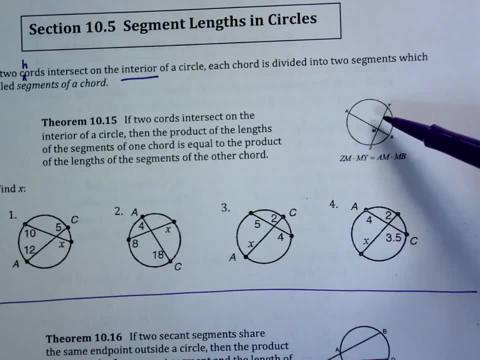 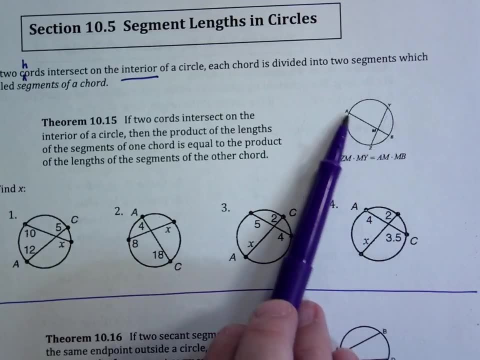 One part over here and one part on the other side of the chord it crosses, And this one too, Chord AB. it's kind of hard to read the letters, but that's A, that's B. Chord AB is divided into two parts: A to M and M to B. 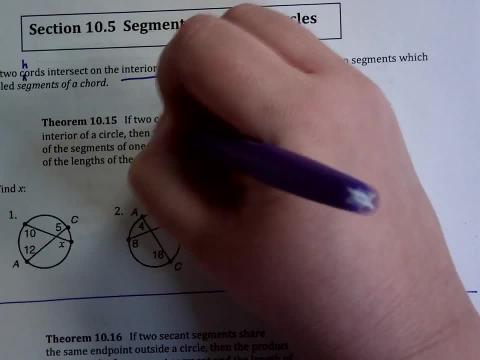 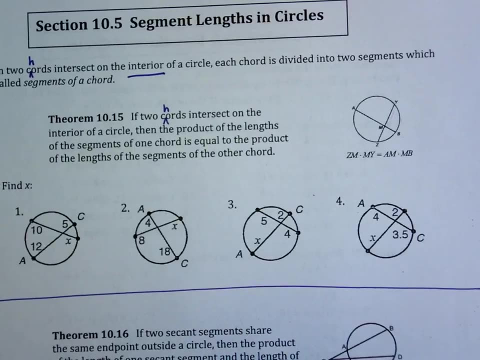 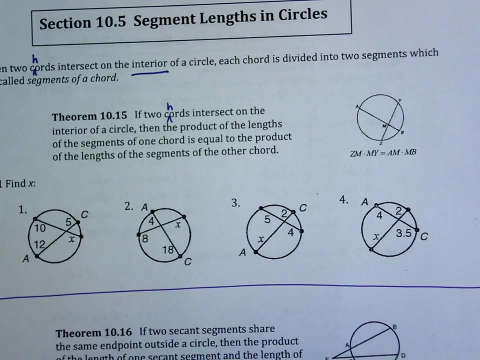 Okay, Okay. So if two chords with an H intersect on the interior of a circle, then the product of the lengths of the segments of one chord is equal to the product of the lengths of the segments of the other chord. That can be a little bit hard to wrap your head around what they're saying. 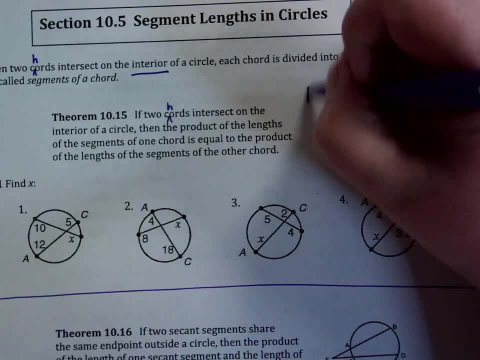 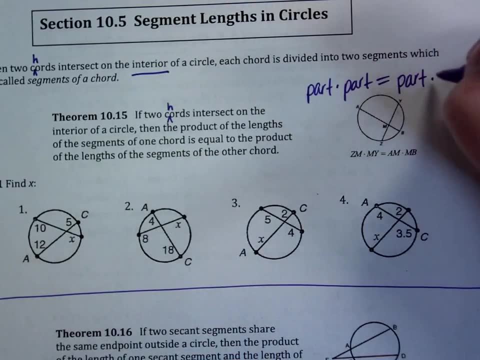 So here's how we like to say it. We like to say, basically, part times part of one of the chords equals part times part of the other chord. So this is how I will say it to kind of help remember it. 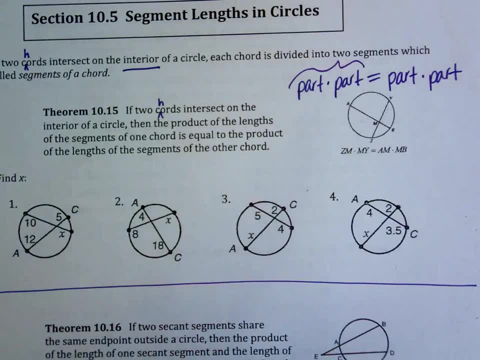 Now, all of the chords are equal parts. All of these. these are all of one of chords and these are all of the other chord. So it's not like I mix and match part of one chord and part of another chord. 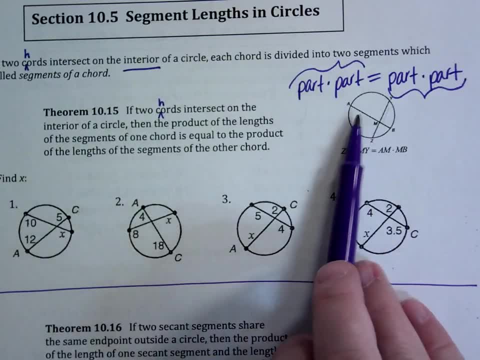 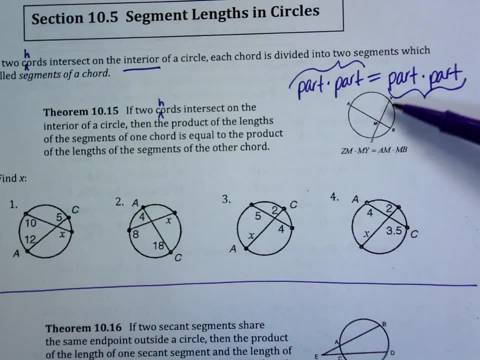 It's two parts of the same chord, So in other words, A, M and M B get multiplied to each other, And then on this one this says Y M Z, So the chord is Y Z. 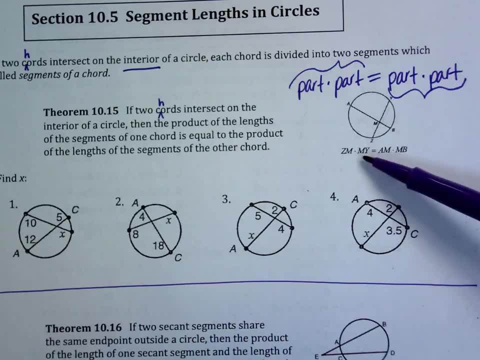 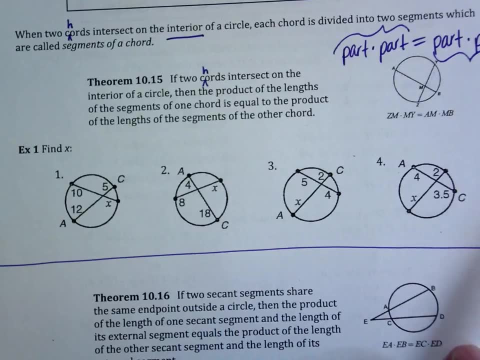 The two parts of chord Y, Z, Y, M and Z M get multiplied times each other. So for example, one The 10 is going to get multiplied by the what The X, the other part of that same chord. 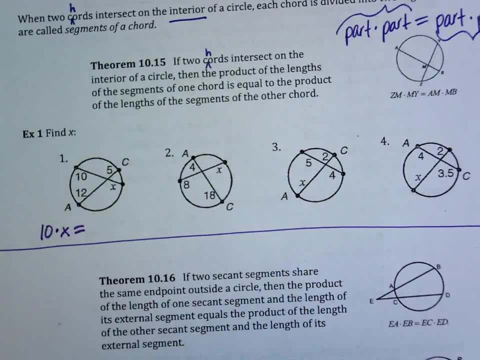 So 10 times X equals what times what? 12 times 5.. There you go, So 10 times X. I should have drawn my line a little bit lower. I'd like some space here, but I didn't. 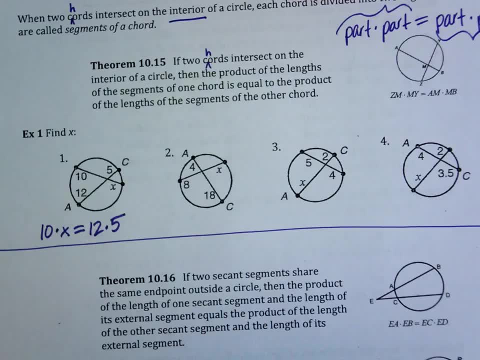 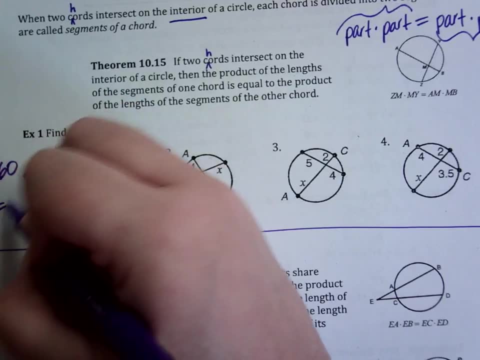 10 times X equals 12 times 5.. What's 12 times 5? 60.. So if 10X equals 60, let's go over here. X equals 6.. Oh, can't see it very well. 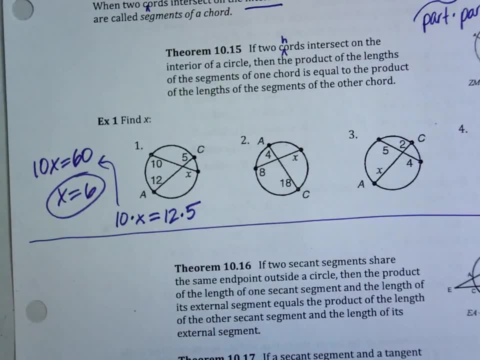 Sorry, All right, Number 2.. What does the 8 get multiplied by X? So X 8 times X, which is just 8X, equals. what does the 4 get multiplied by 18. 18.. 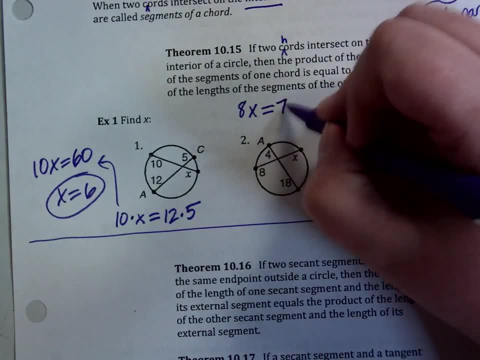 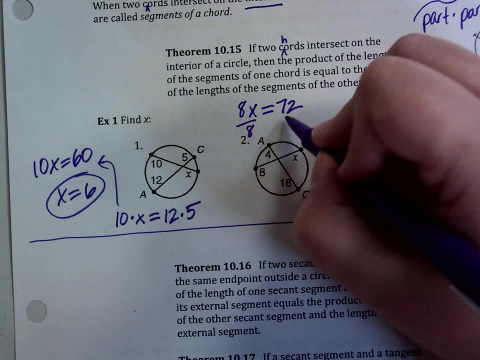 What's 4 times 18? 72.. 72 is correct. Then what Divide by 9.. Divide by 9. By 9? Not 9. 8. That's my bad. X equals 9. All right. 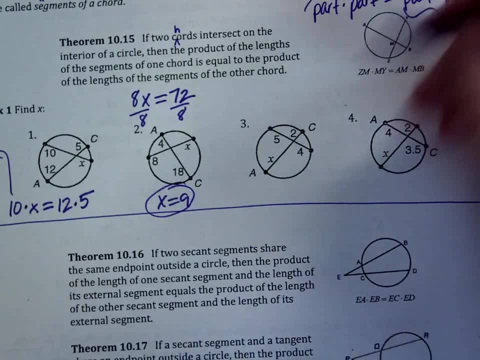 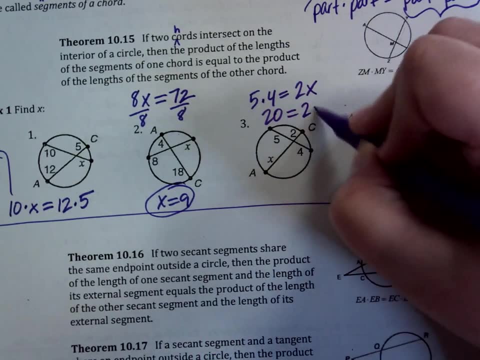 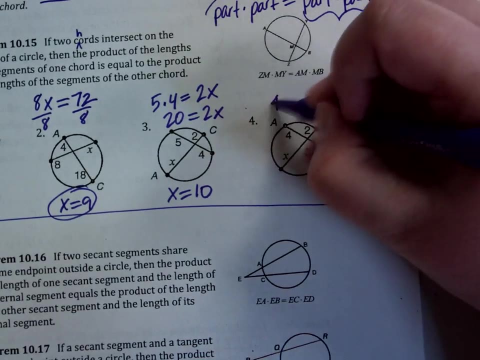 Next one: 5 times 4 equals 2X. 5 times 4 is 20.. So if 2X equals 20, what's X? 10. 10. And last but not least, 4 times equals 2 times 4.. 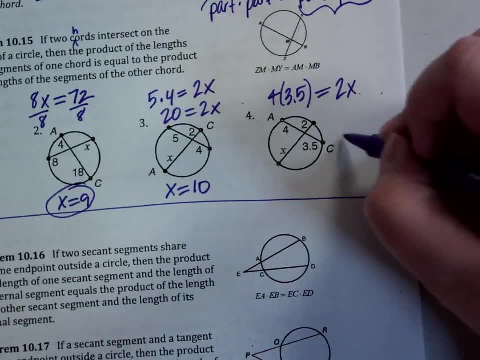 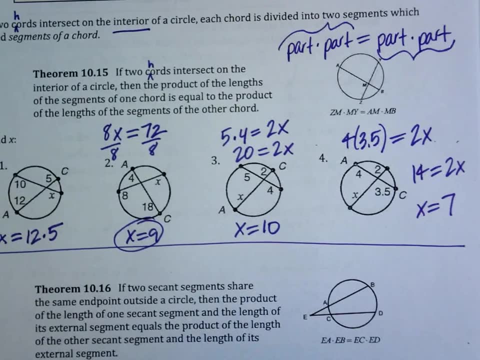 4 times 3.5 is 14.. 14 equals 2X, X equals 7.. Ta-da, That's all you have to do for those. So these are chords that intersect in a circle, and these are the pieces of their lengths. 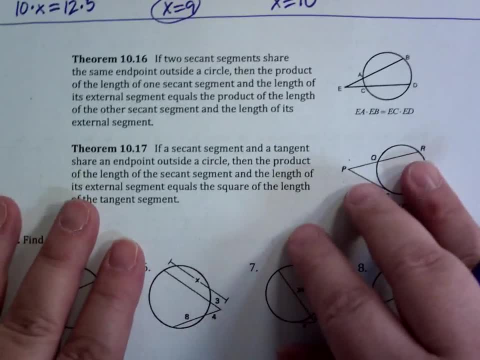 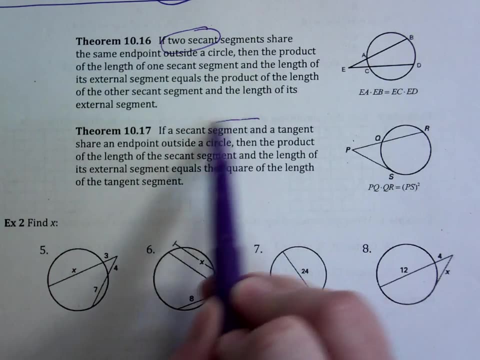 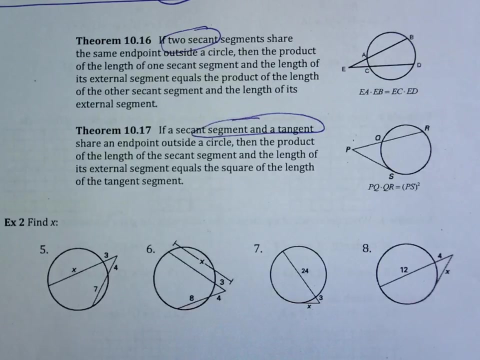 All right. Next relationship: Notice that they have two theorems here. One of them is if you have two secants, and the other one is if you have one secant and one tangent. Okay, Okay, So I'm going to combine them into one rule. 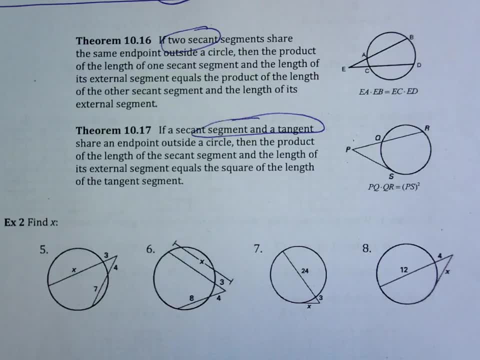 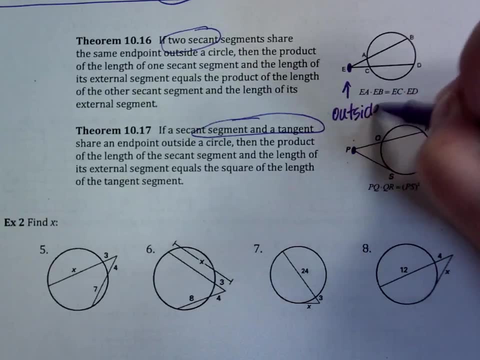 I'm going to just say there's one rule, because notice that the thing they have in common is both of them. the segments intersect outside the circle. That's what they have in common. So we're going to have one rule for inside. 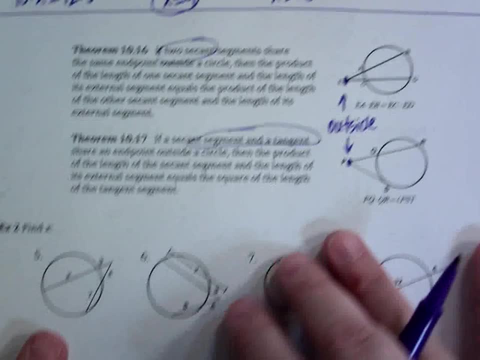 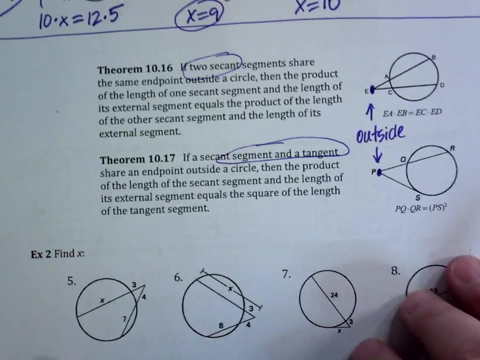 We already did it up here. We're going to have another rule for outside. Now the special case gets a little bit different, but I'll show you that when we get to it. So our rule for outside is going to be: where do I write it? 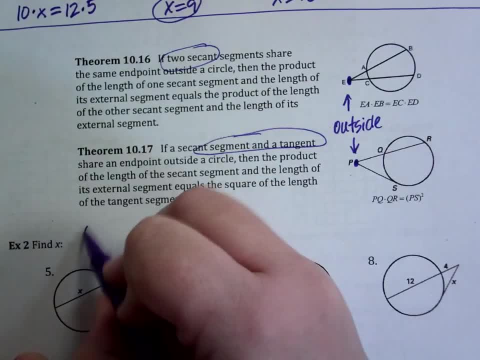 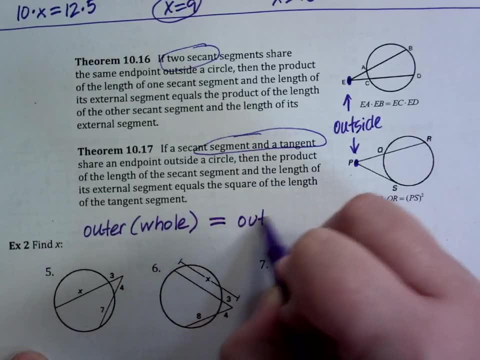 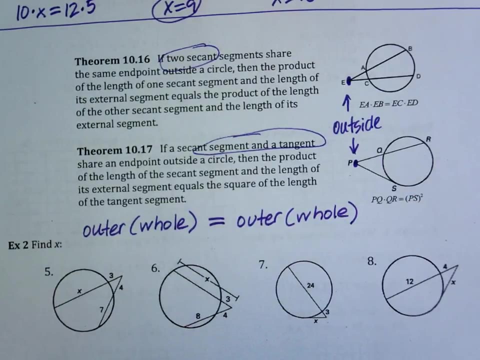 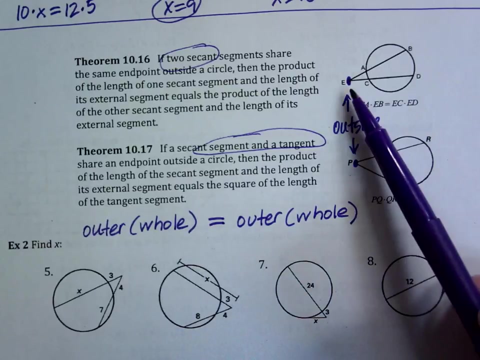 I'm going to write it right here That the outer part times the whole thing on one segment equals the outer part times the whole thing on the other segment. So write that down. So on this top the outer part means EB is the whole thing. 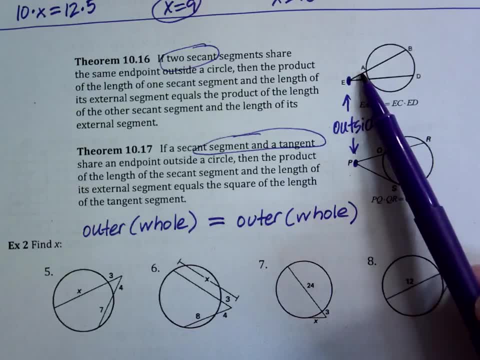 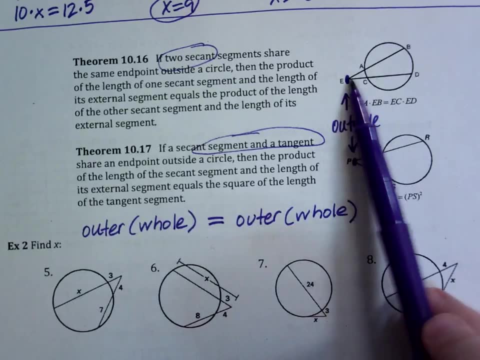 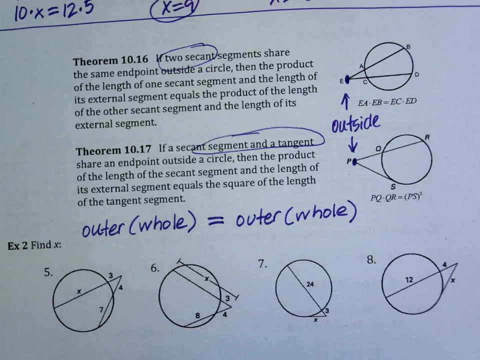 So the outer part of EB is just EA. Okay, So EA times EB. See that EA times EB. And then the other segment that comes from E: the outer part is EC and the whole thing is ED. Notice that the whole thing includes the outer part. 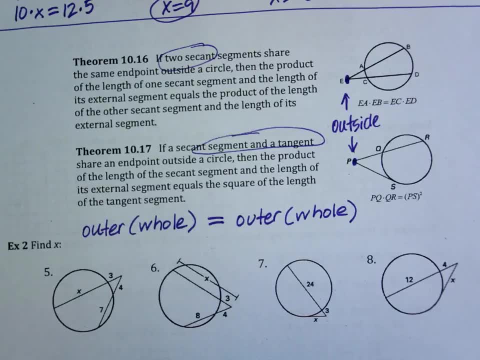 So it's outer part plus inner part. Sometimes that will come up because you'll have to add with variables. On this example, here, outer part for PR is just PQ. Okay, Whole thing is PR. So that's here. 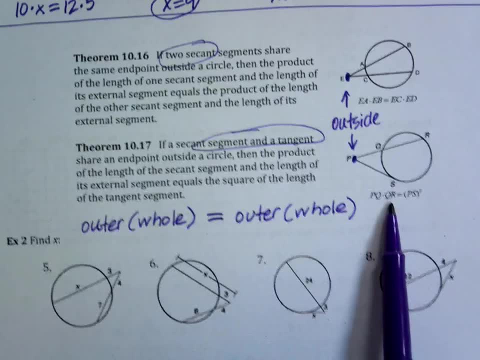 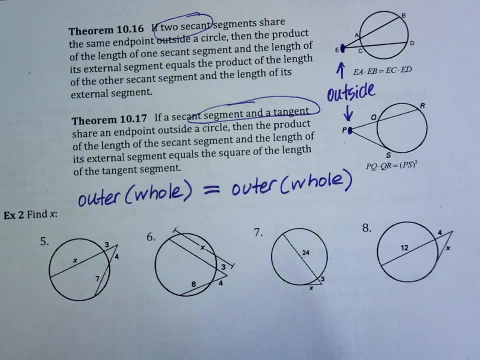 Now notice on the other one, the tangent segment, the outer part is the whole thing. When the outer part is the whole thing, that means it just gets multiplied times itself. Outer part is PS, Whole thing is PS, So it's just PS times PS, which is PS squared. 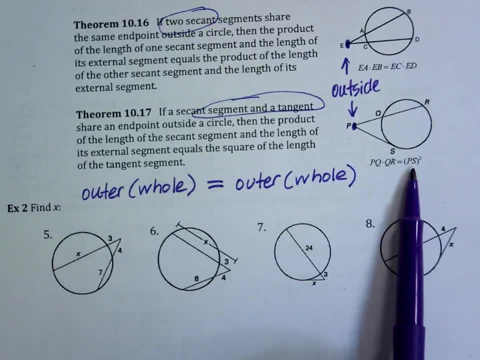 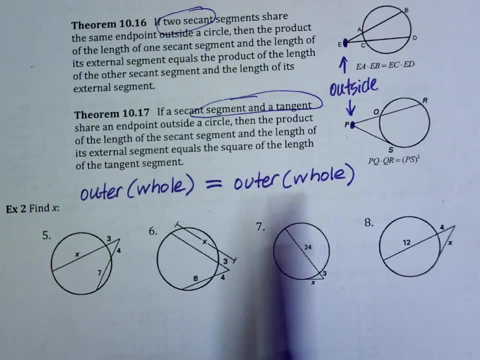 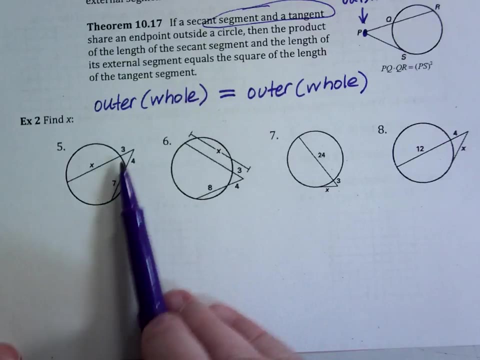 So that's the difference is that for a tangent, you just have to remember that on one of them the outer part will be the whole thing, And so you just multiply it times itself. All right. So for instance, on number five here, this segment up here, what is the outer part? 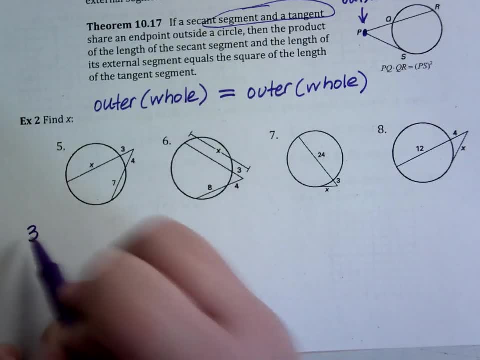 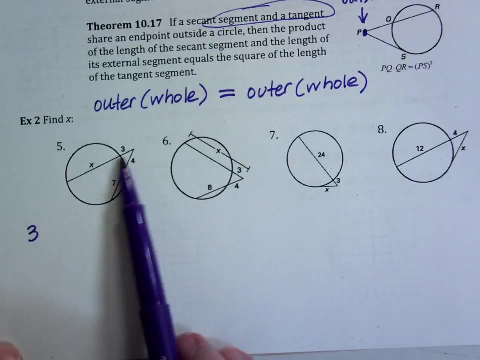 Three, Three. Now here is the thing I told you guys about this in the last unit. There is a temptation to call the whole length here 3X. It is not 3X. What is it? X plus 3.. 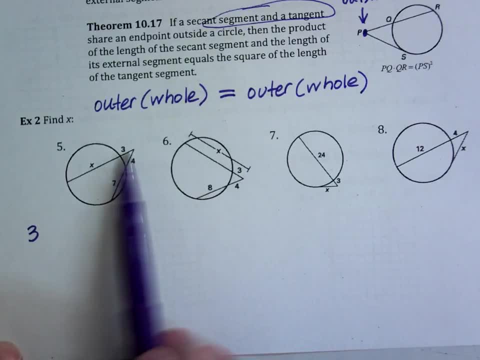 It's 3 plus X or X plus 3.. When you're doing two parts of a segment and putting them together for a whole length, it's 3X. Okay, When you're doing two parts of a segment and putting them together for a whole length. 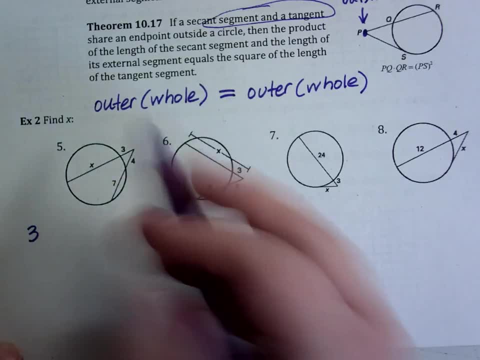 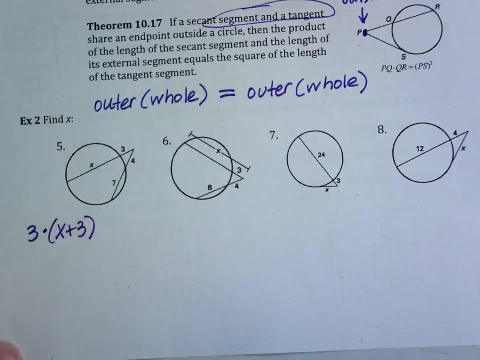 you add them, Don't multiply. So this is not going to be times 3X, It's going to be times 3 plus X. So or we're going to call it X plus 3.. You have to distribute. 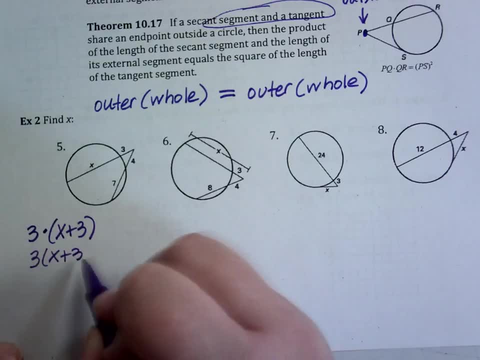 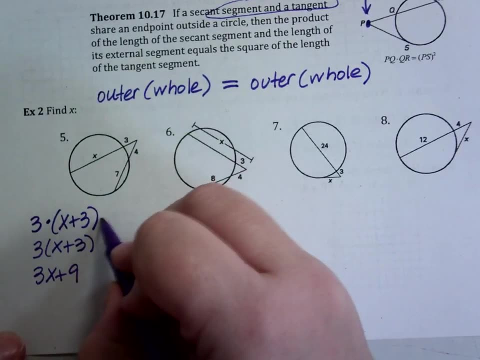 This is the same as this. So on this side of my equation I'm going to have 3X plus 9.. On the other side, the outer part is 4.. What's the whole thing? 4 plus 7.. 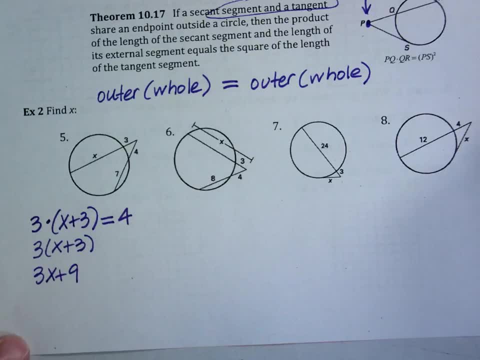 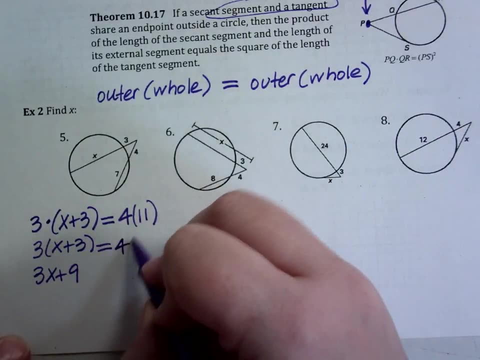 Okay, What's 7 plus 4? 11.- 11.. Make sure you're adding again: You wouldn't multiply the other side. You don't multiply the other side, So that's 44.. So that's 44.. 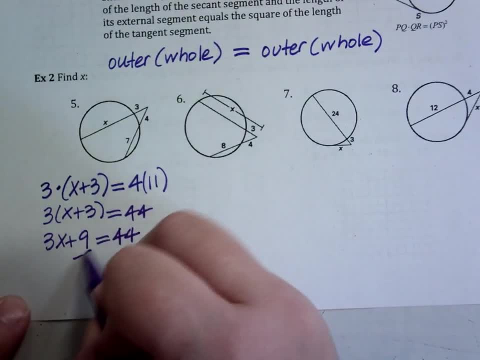 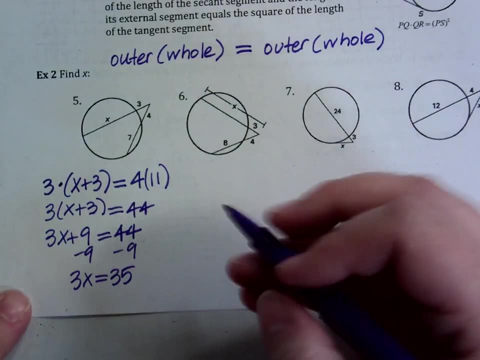 And now I can solve my equation: Subtract 9 from both sides, 3X equals 35. Is that right? Yup, Yup. So that means it's not going to come out exactly, So I would probably just leave it like this. 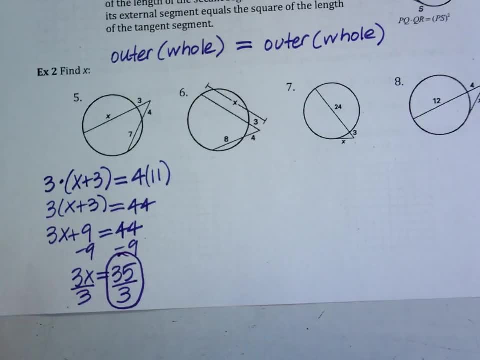 It's not going to come out as a whole number. That's what I meant by exactly. Okay, It is exactly, It's just not whole. Now I want you to notice that number 6, things are written a little differently. 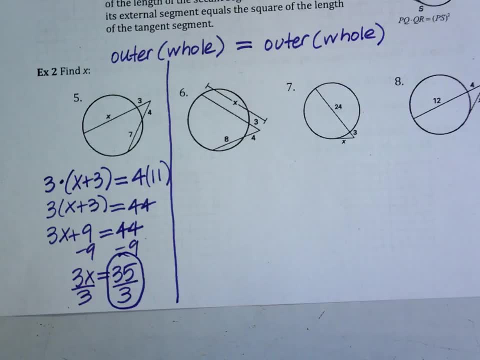 You have to notice when it's given to you differently. What's different? The whole thing is X. The whole thing is X. You don't do any adding to get the whole thing, because they're telling me that the whole thing is X. 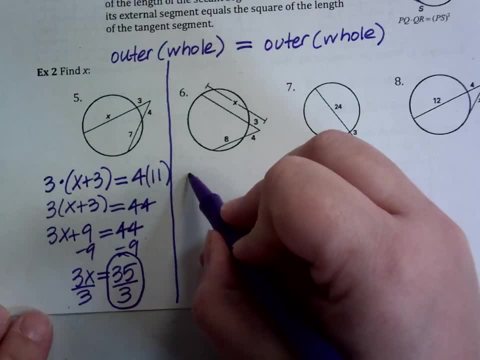 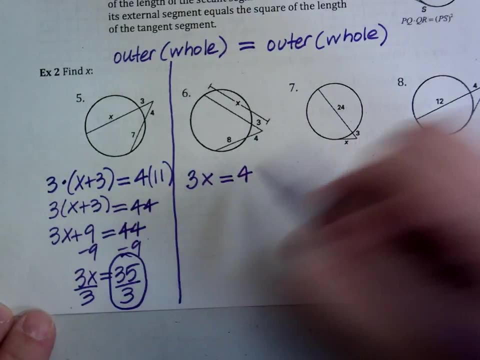 So on that segment, outer part is 3.. Whole thing is X, X And on the other segment, the outer part is 4 and the whole thing is 12.. 12. Where'd you get 12?? 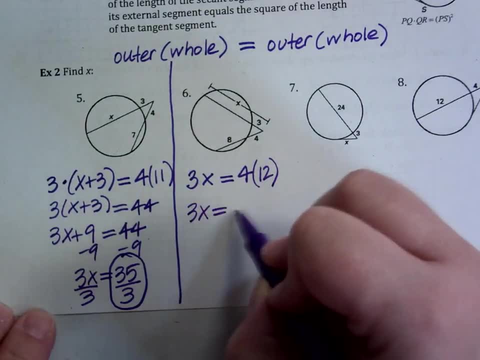 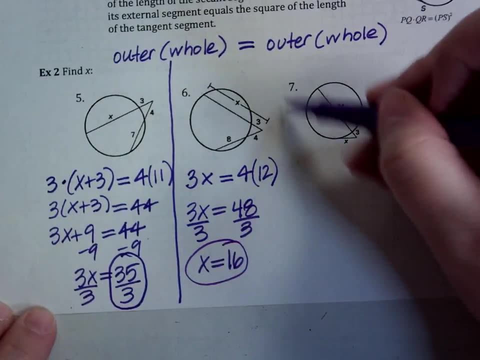 Adding 4 plus 8.. 4.. 4 plus 8.. You got it. So this gives me 48.. And X is 2. 2.. Good, All right. Next Let's go with the tiny segment. first. 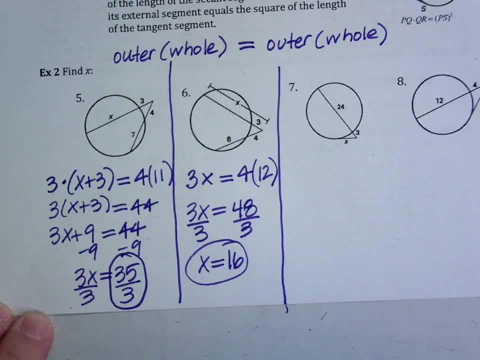 It's a tangent segment. So what's the outer part of that segment? X, X, Y'all are jumping ahead. The outer part is X, The whole thing is X, And so that's why you just said X, squared. 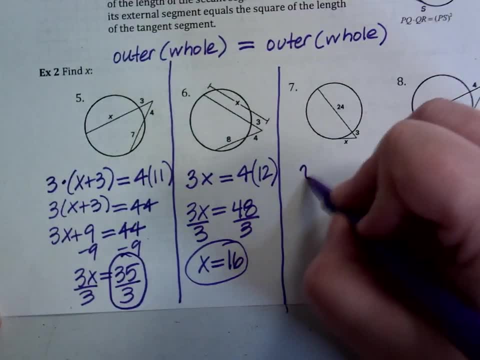 X squared Because it's the outer part times. the whole thing is just going to be X squared. So X squared equals 3 times what 27.. 27. Not 24. Be careful to add it. So X squared equals 81.. 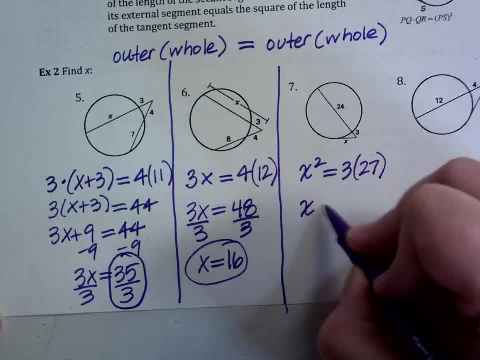 So what's X, 9. 9.. Is this a case where it could be plus or minus 9?? Yes, Yes, Well, actually, No, I'm going to go with your – well, actually, Dillion. 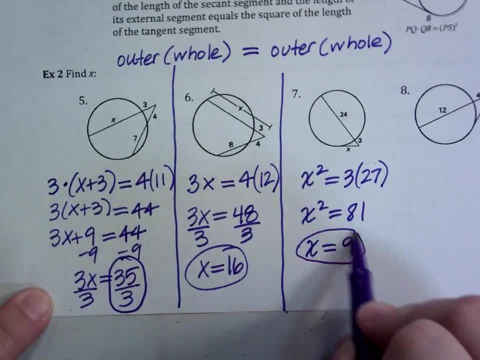 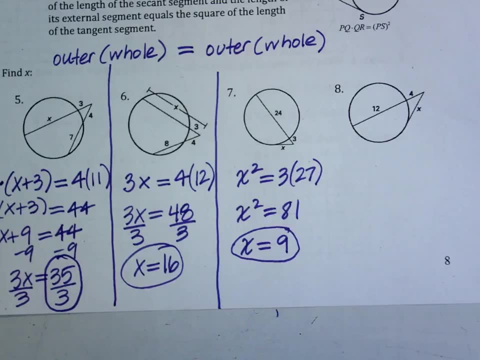 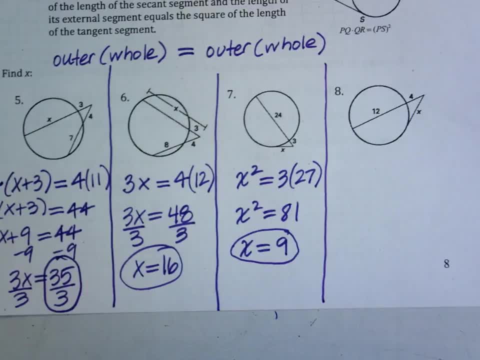 So it has to be positive 9.. That's why I didn't put plus or minus, All right. Last but not least, tell me how to set this one up, Starting with the X. X squared equals 4. 4.. 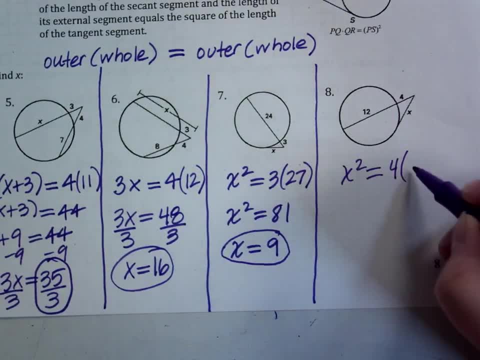 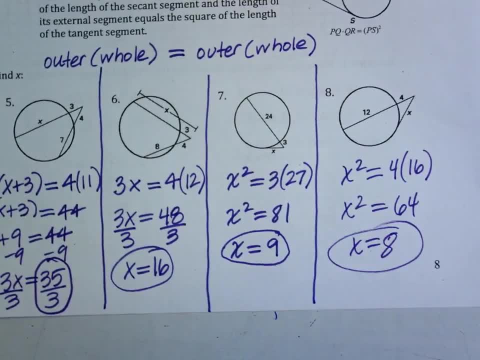 8., 8. You are perfect, Ta-da. Good job. Say bye everybody, Adios, Bye. Wait. I'm sorry, We have one question. What's the question Like on the example? it says: like PQ times PR. 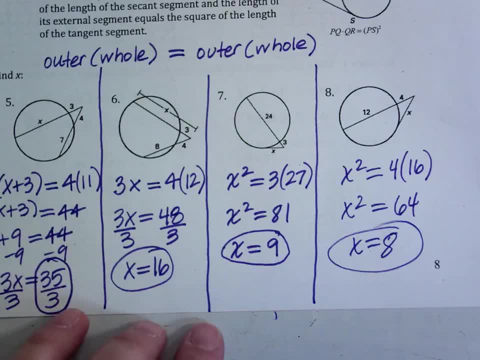 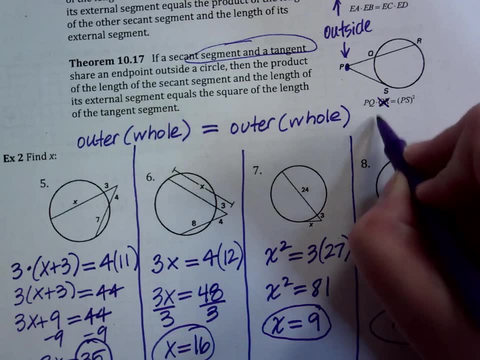 Yeah. Oh gosh, That's terrible. They're wrong. Okay, Uh-huh, So it's PQ times, PR. Yeah, This should say PR. Okay, Yeah, Absolutely, Thank you, That was wrong, I promise. 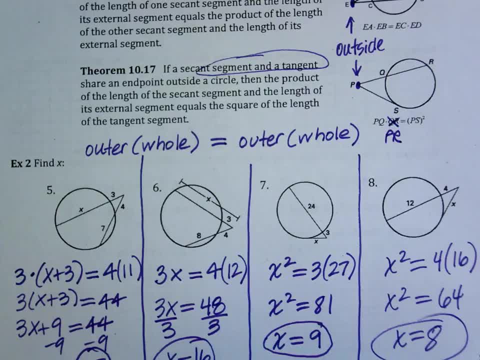 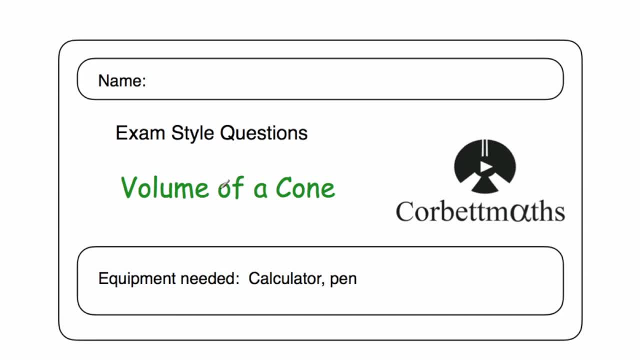 Hi, welcome to this CorpMaths video. In this video we're going to look at the video solutions to the volume of a cone- practice questions. If you need any extra help on finding the volume of a cone, if you go to CorpMathscom forward, slash contents. 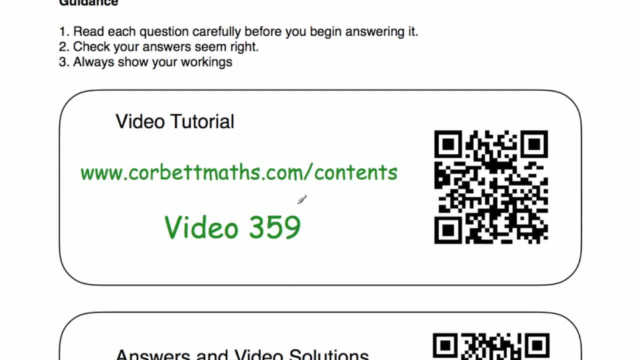 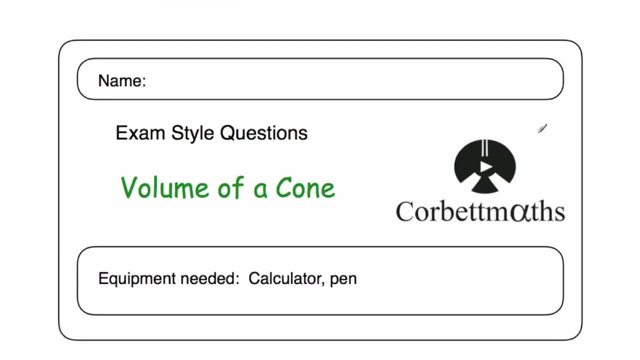 there's a video tutorial there- video 359, that shows you how to find the volume of a cone and answer typical questions on it. Alternatively, you could scan this QR code and it will bring you straight to that video. In this video, we're going to be focusing on the video solutions to the answers to the practice questions.